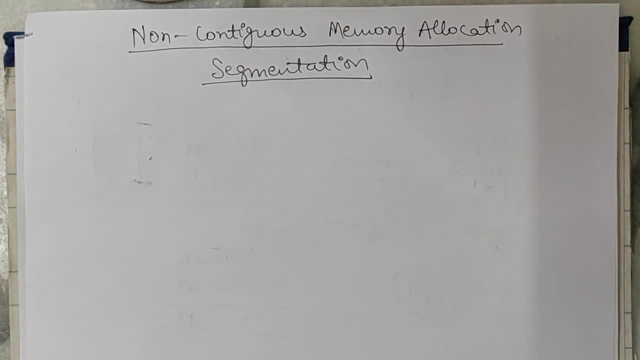 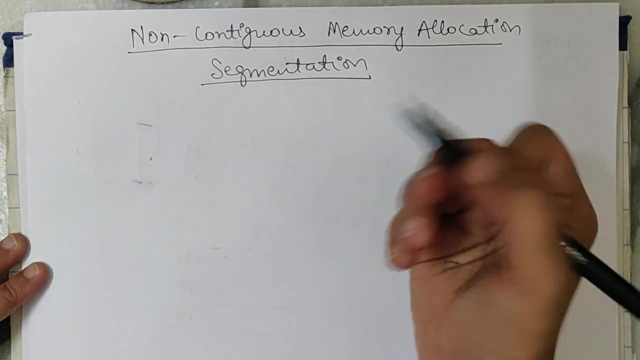 Hello everyone, welcome to operating system tutorial. In this tutorial, I will discuss the non-contiguous memory allocation technique which is segmentation. There are two techniques: one is paging and other is segmentation. I have already discussed paging in my previous videos, So in this video I will discuss segmentation. So let's get started. So segmentation. 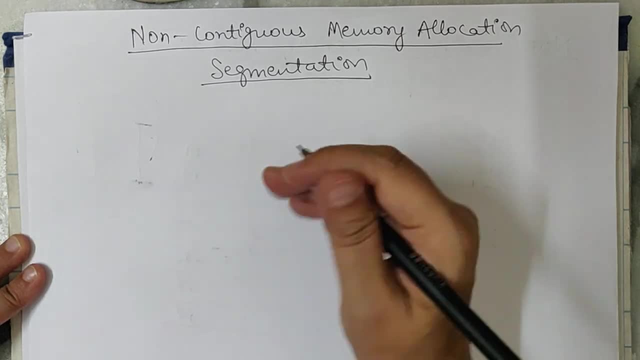 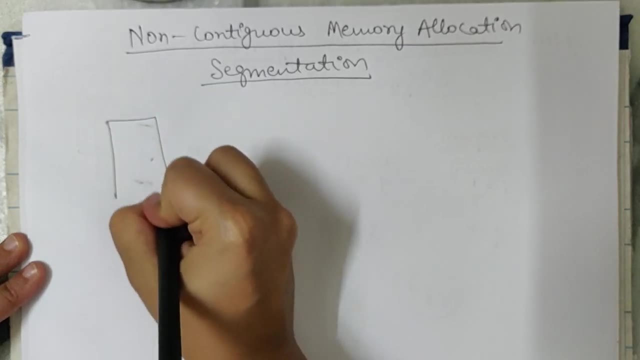 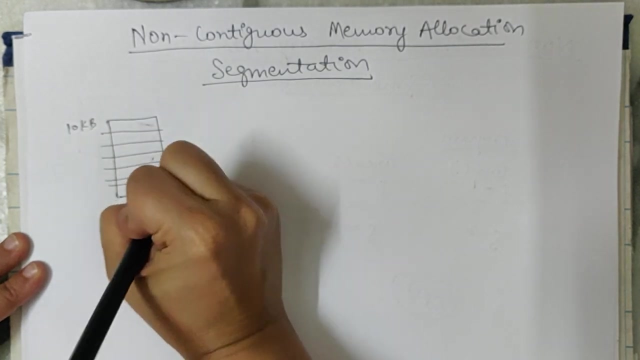 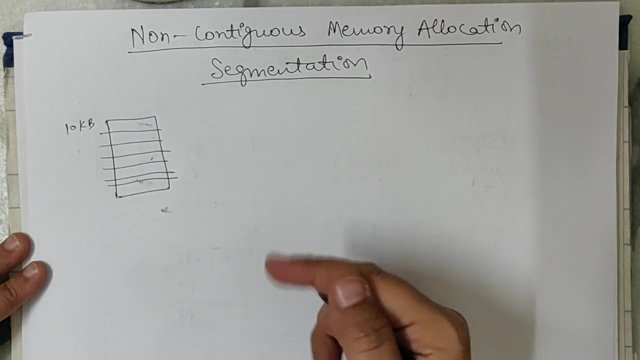 is basically in paging. we have to cut our program into equal sizes. This is our program of 10 KB. We have cut 10 pieces of 10 KB program and each piece is of 1 KB. We have cut equal size pieces. We used to do this in paging. Now, what is the problem with paging, Say? 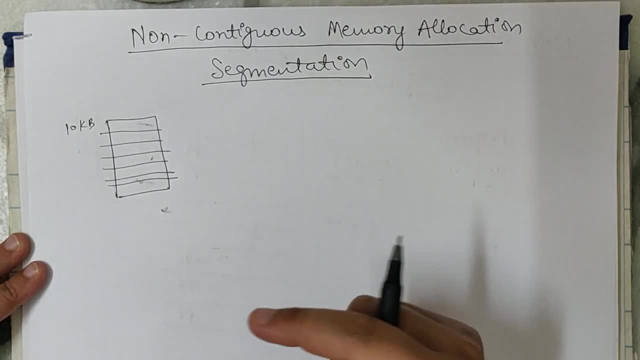 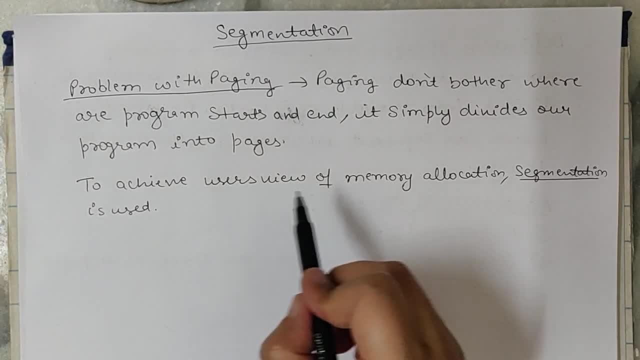 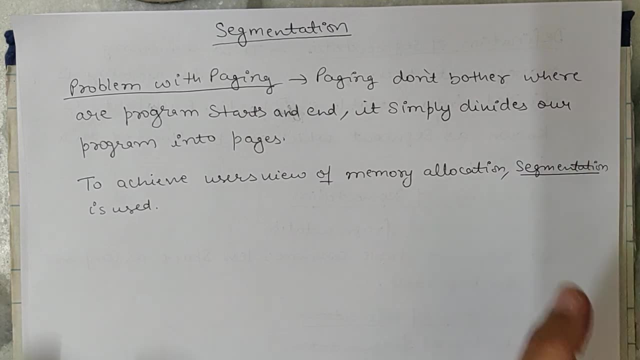 cut. So we have to make a program which we have to cut. So we have to make a program which we have to cut. So we have to make a program which we have to cut. So we have to figure out which is. 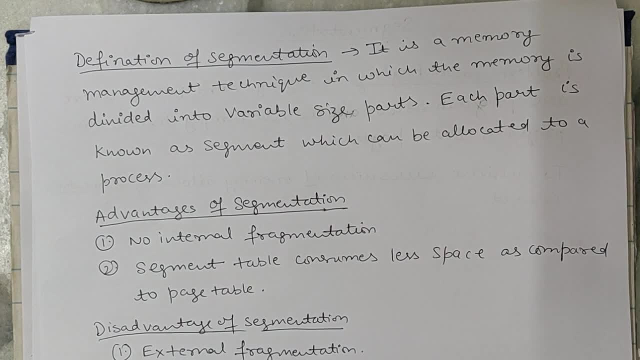 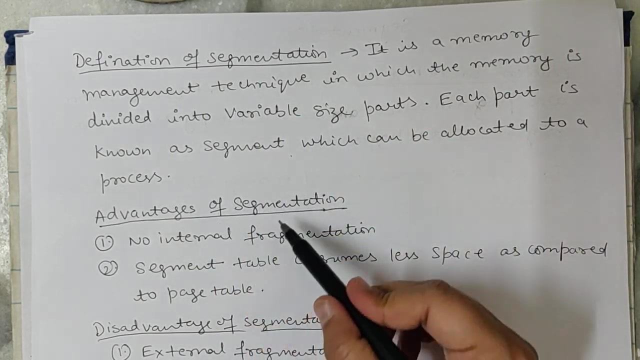 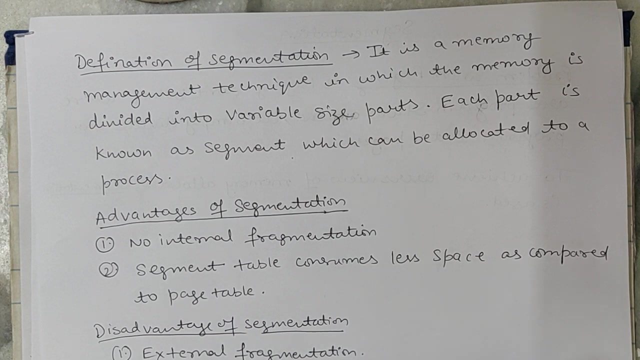 the metric, Then we will be reporting the the, the metric, Then we will be reporting the metric. Then we will be reporting the advantages and these are some disadvantages: that there will be no internal fragmentation but it can be external, because we are doing partitions in pieces according to ourselves. 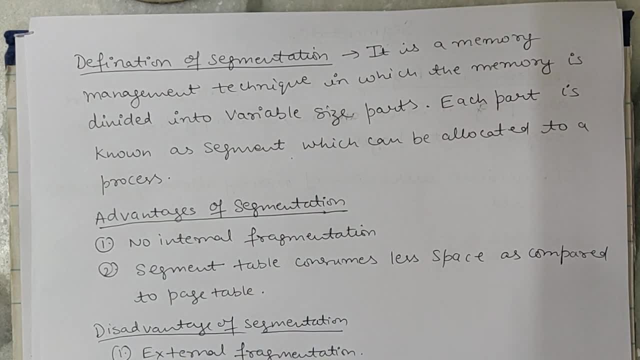 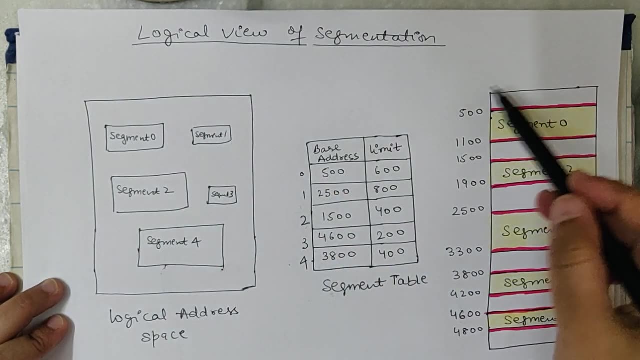 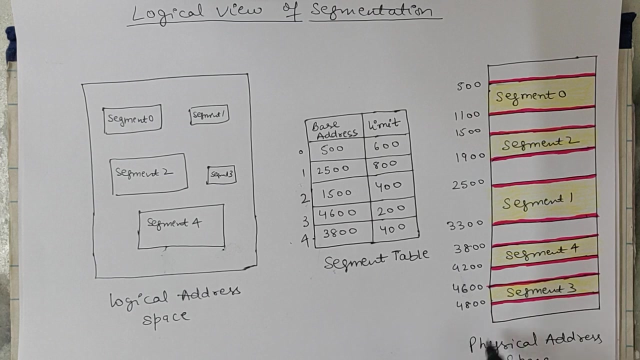 so there are chances of external fragmentation, but there are no chances of internal fragmentation. now let's see this logical view of segmentation. this is my secondary memory and this is my main memory. in main memory the addresses are physical addresses and we called it physical address space and in physical memory. 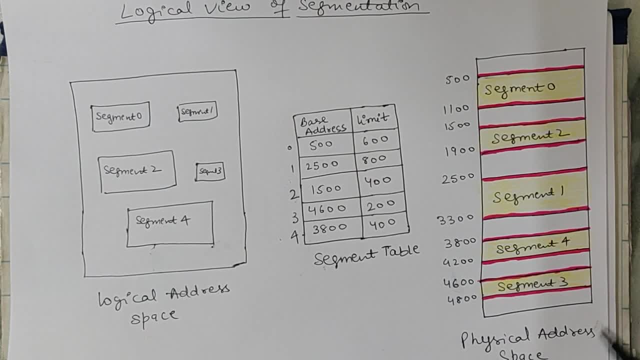 the addresses in main memory are physical addresses and collection of these addresses is physical address space and this is my secondary memory. and in secondary memory there are logical addresses and we named many logical addresses, logical address space. this is secondary memory and this is main memory. so we are just seeing its view. 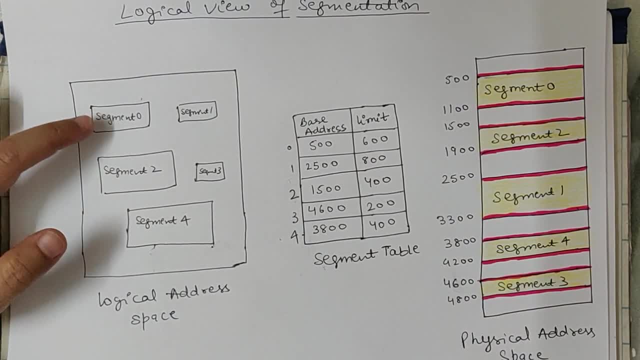 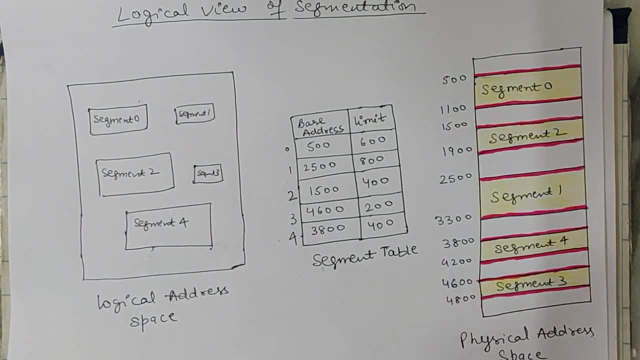 that how segmentation happens. so suppose this segment is zero, like this: we have 4 segments, we have 5 segments: segment 0, segment 1, segment 2, segment 3, segment 4. now in every segment there will be number of instructions. 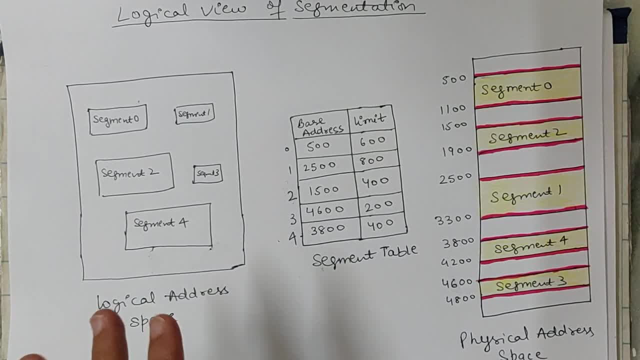 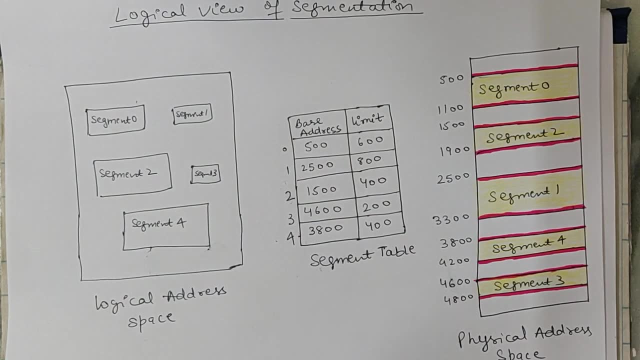 code will be written and each one's size is different. each one's size is different and each one will have some length. each segment will have some length. length means there will be number of instructions, but it is not necessary that it is same. in paging it is same, but it is not necessary. 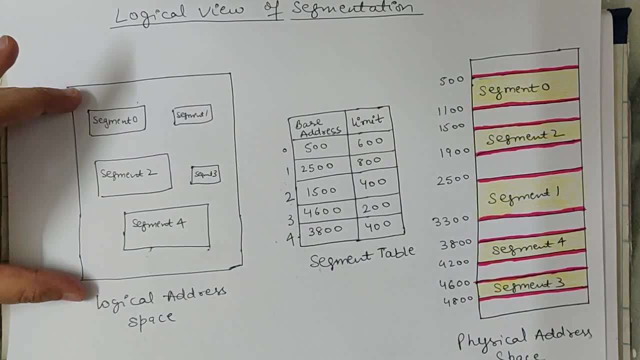 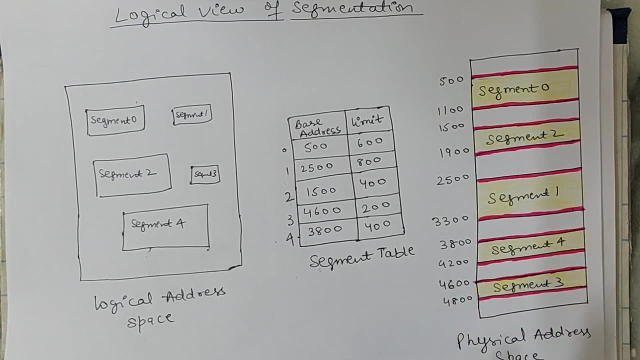 so this segment we have kept it in secondary memory, like in paging. like in paging there is page table, like in segment there is segment table. every process has its own segment table. suppose this is our process x. so in process x we have cut pieces in 5 segments. 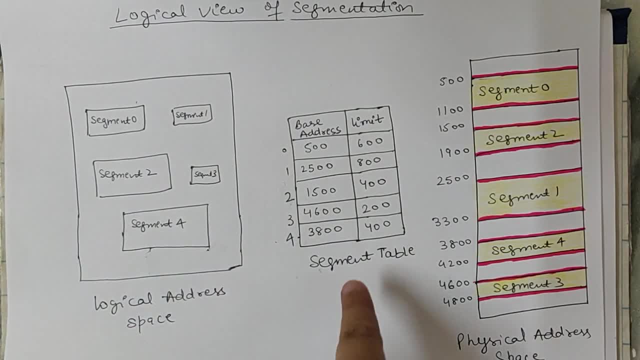 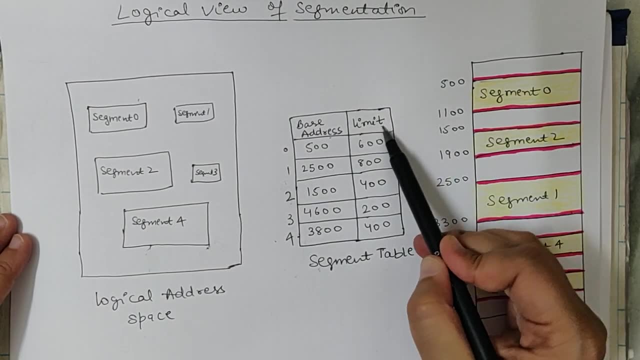 segment 0,, 1,, 2,, 3,, 4 and in process x there is segment table and in segment table there are 2 fields: base address and limit. what is the meaning of base address, that particular segment number 0, segment 0? 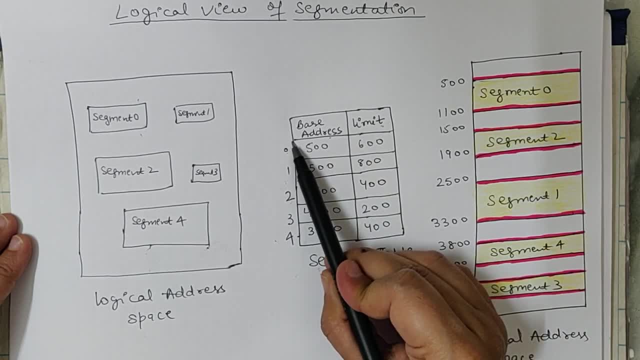 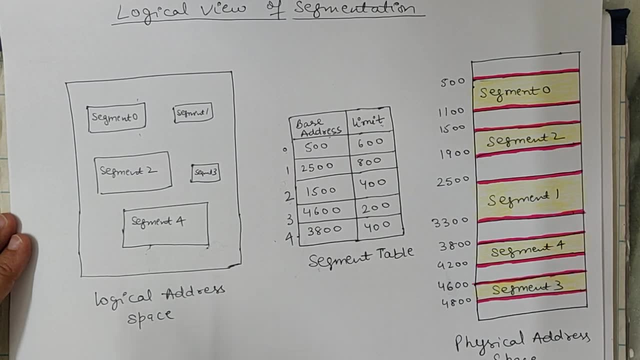 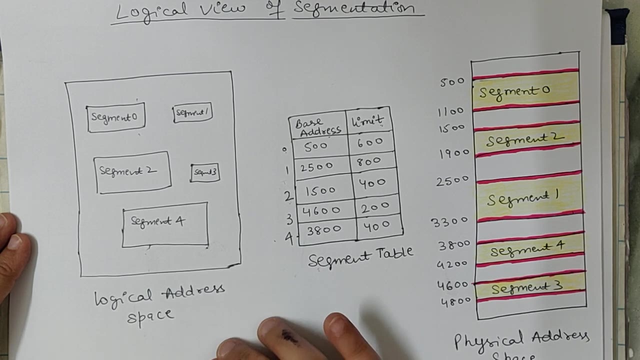 in main memory from where it is starting and how much range it has. limit means how much number of instructions it has. ok, so now you forget this. ok, forget this now. we are just seeing that our process number is x. we have made 5 pieces of it. 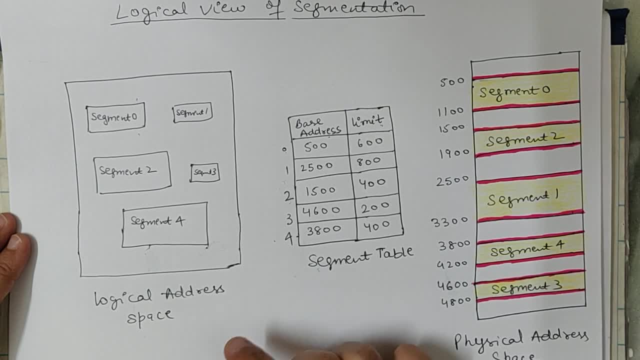 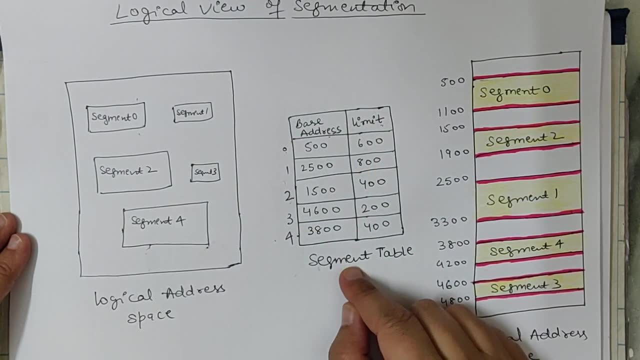 every piece we have cut in different size and every piece's name is segment 0,, 1,, 2,, 3,, 4, ok, and we have made a segment table of process x- we will not see this now- and every segment segment table has 2 fields. 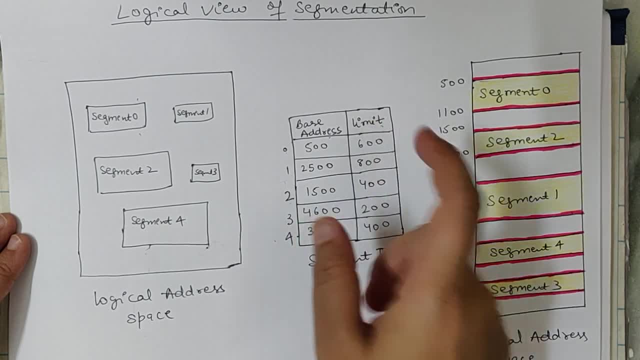 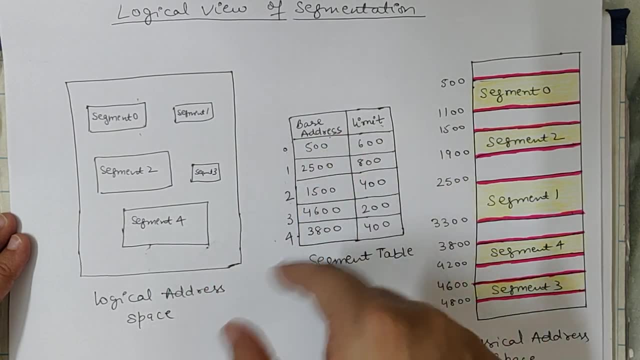 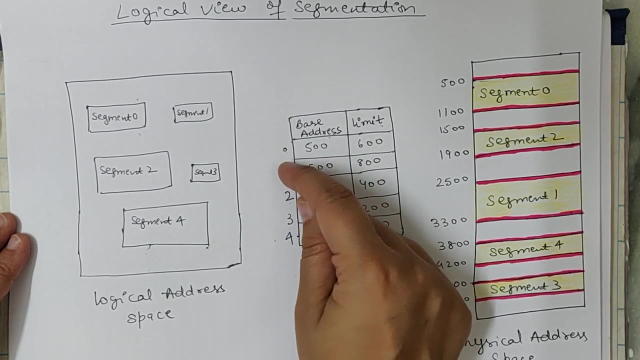 first field is base address. second is limit. limit means how many number of instructions it has per segment, how many instructions it has segment 0 in main memory. what is the base address of segment 0 means from where segment 0 is starting, from which address it is starting. 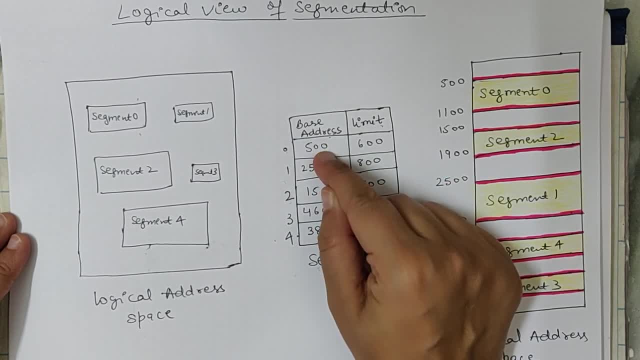 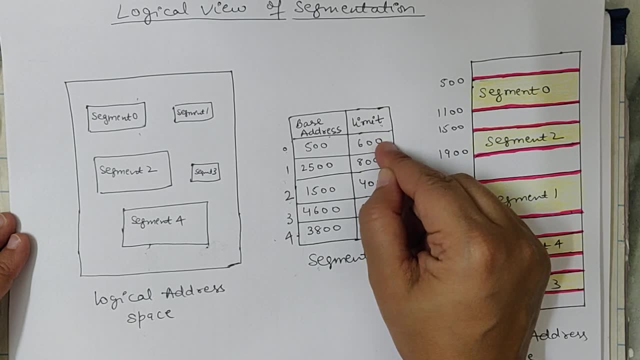 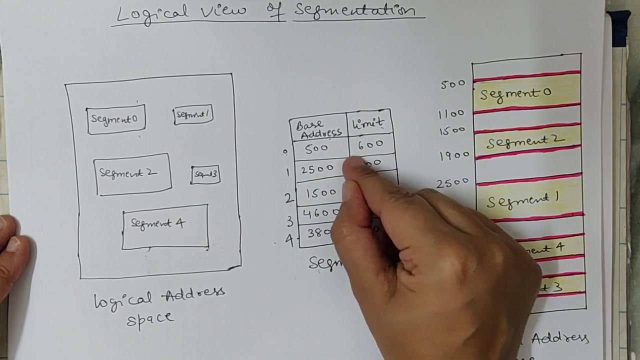 and how many instructions it has. so it is starting from 500 and its range limit means how much range it has. how big is the segment? it is a segment of 600 instructions. segment number 1 is starting in main memory from 2500 and its range is: 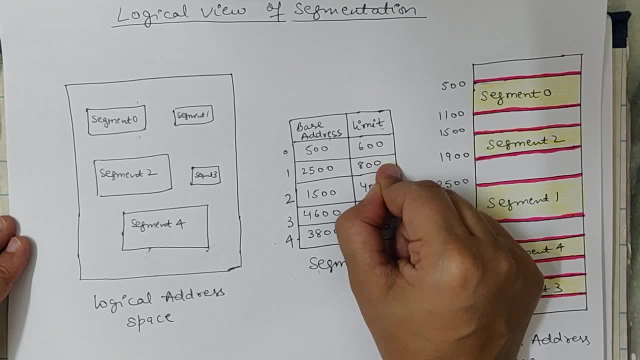 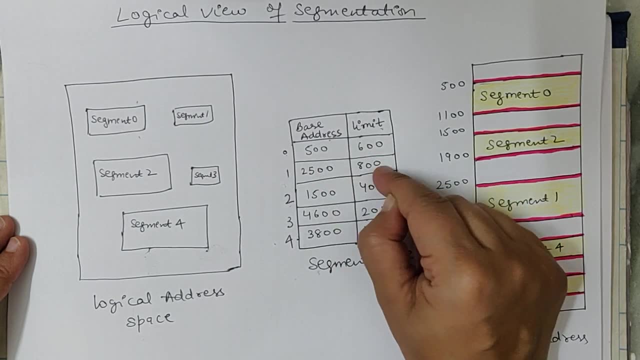 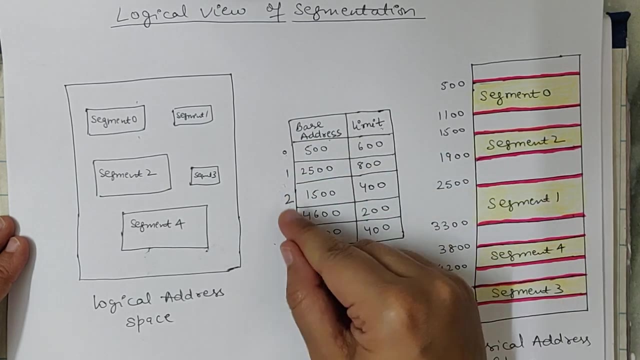 instructions are 800. its size is basically size of the segment. limit means size of the segment. first segment's size is 600, second is 800. and what is this? from where it is starting in main memory? in main memory, from where is that segment starting? segment number 2: 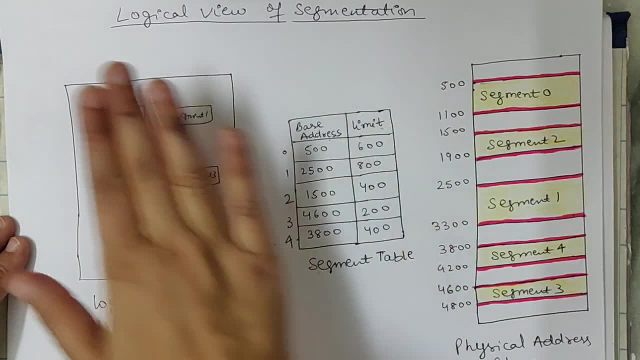 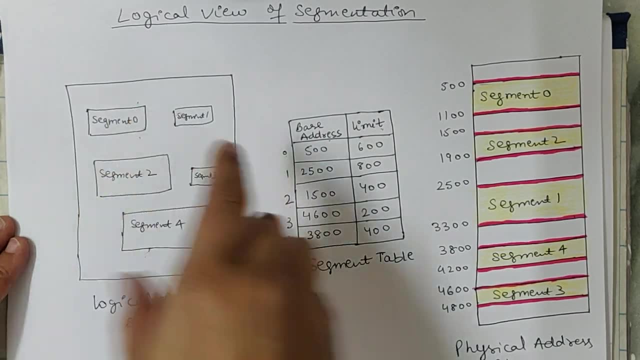 is starting from here. segment 3, segment 4: now all these segments are loaded in main memory. ok, as it is. so segment. now what will happen? segment 0: from where is it starting? from main memory, from 500, and its size of first segment is 600. 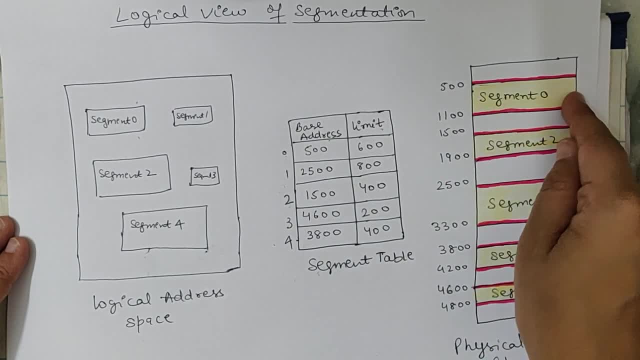 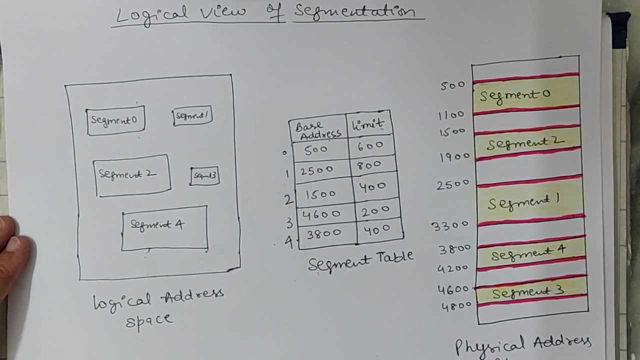 so 500 plus 600 will go to 1100. so this is denoted segment number 0. ok, now let's come to segment number 1. segment number 1: from where is it starting? now it is read randomly because it is a non-contiguous. 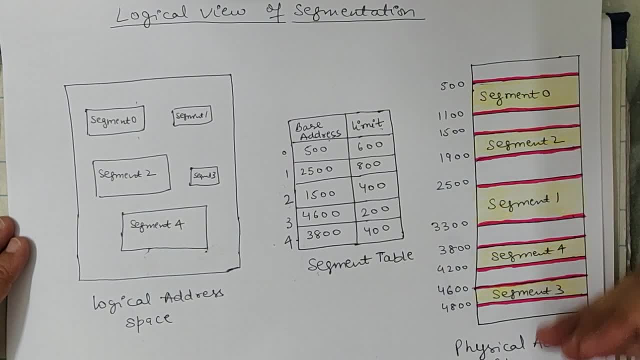 memory allocation technique, so it is not necessary that all the segments will be in sequence: segment 0, 1, 2, 3, 4, no, where it is in main memory now this blank space, this means that it will be occupied where I haven't done shade. 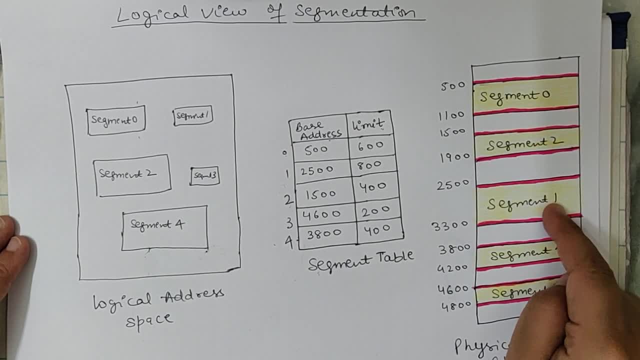 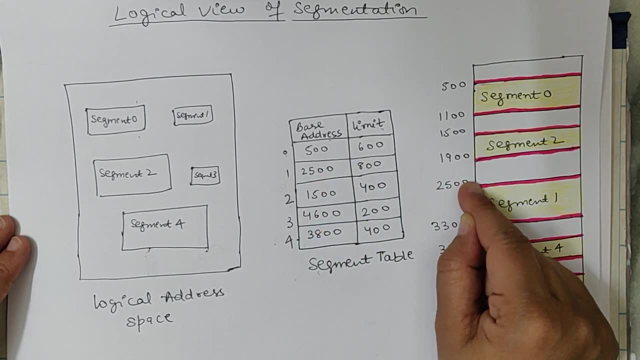 that means it will be occupied somewhere. we can't use it. that's why segment 0 is here. segment 1 is here. so where is segment 1? its base address is 2500, so where is it starting from 2500? how much is its size? 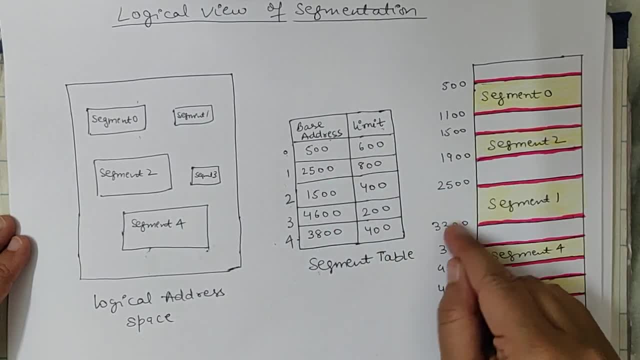 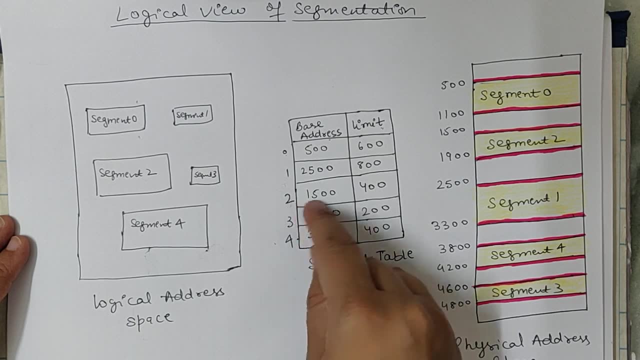 of that segment: 2500 plus 800. so the size, no matter how much it is, 2500 plus 800, it will reach here till 3300. ok, where is segment 2? its base address is 1500, so where is it starting? 1500 plus.